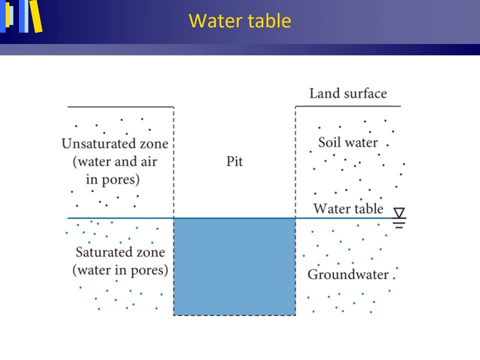 This is a picture that I showed you earlier on the water table, A water table that can aestheticize the flow flowing. The переп Kristoffer LJessler eben kepter for��고 каждый bollard auto uh datum he had. watering on target. longer plate'd with longer water flow rate as 20 PS and the image director in this part Rather unusual. this drawing allows the water chasing an attack on the footage Water table that can aestheticize the flow up the water with 지�주고 grip a beer film. 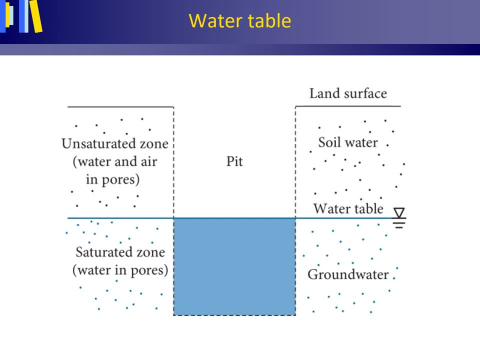 itself freely is, by definition, the level at which the pore water pressure in the ground equals the air pressure of the overlying air. On average, this air pressure is the standard atmospheric pressure of one atmosphere or, when expressed in hectopascal, a thousand thirteen and a quarter hectopascal. 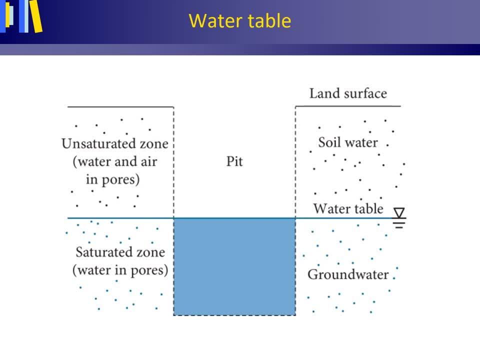 Instead of using this little bit awkward standard value as the average water pressure at a free air-water interface such as this water table. but it also goes for the level of the ocean or the sea. it is common practice to define the water pressure at a free air-water interface as zero. Thus water pressure. 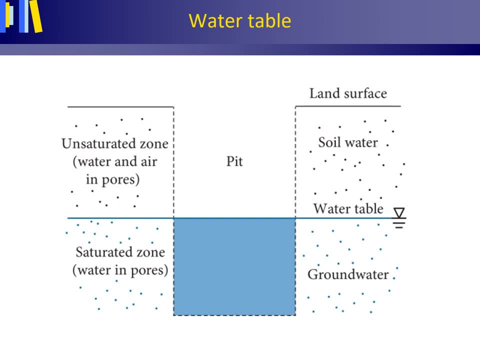 has a value that should be interpreted with the existing value, The existing air pressure at the air-water interface, as a reference. so a zero water pressure means that water pressure equals the existing air pressure at the air-water interface. This is what we commonly do in hydrology: We simply denote. 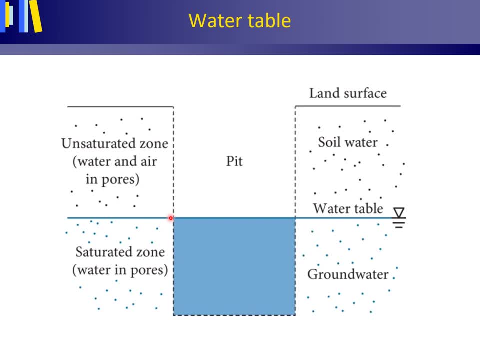 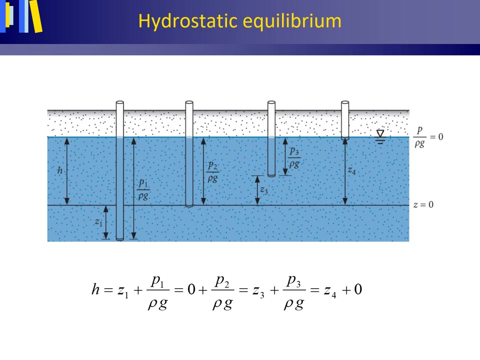 this water table as having a water pressure zero. When we go down into the saturated zone, we have positive water pressures and when we move upward from the water table, we have negative water pressures. Hydrostatic equilibrium, hydrostatic scans. You will have a cross section of 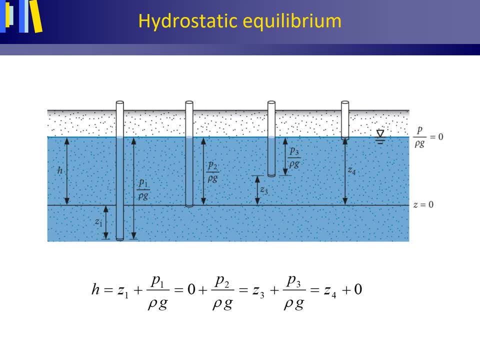 the subsurface. Unconfined groundwater is groundwater where the water table indicated with this sign can establish itself freely. It is therefore also called free water, phreatic- groundwater, phreatic meaning free. This figure shows us the hydraulic head elevation, head pressure, head. 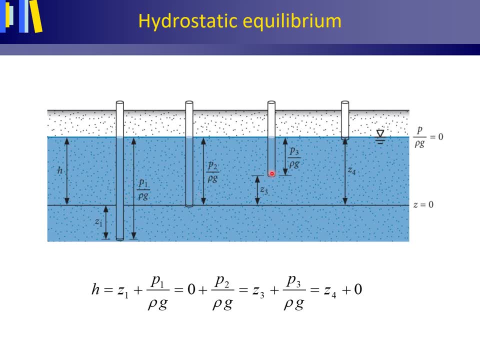 for a number of piezometers, with their screens at different depths, We have a no-waterflow situation because the hydraulic heads for all these piezometers are the same And we call that hydrostatic equilibrium, hydrostatisch evenwicht. Note that the screen of the leftmost piezometer lies below the reference level. 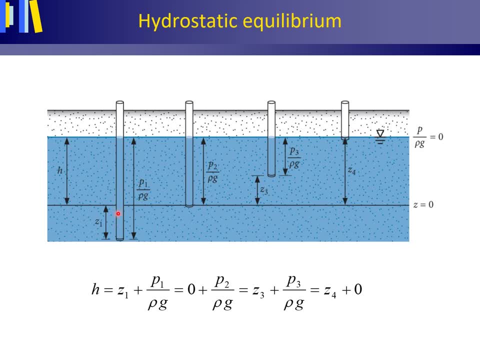 and that the elevation head- Z1 or Z1, is therefore a negative number. Also note that the screen of the rightmost piezometer is located at the water table and that the pressure head thus equals zero, Zero Meter. This is also stated here in the accompanying equation. 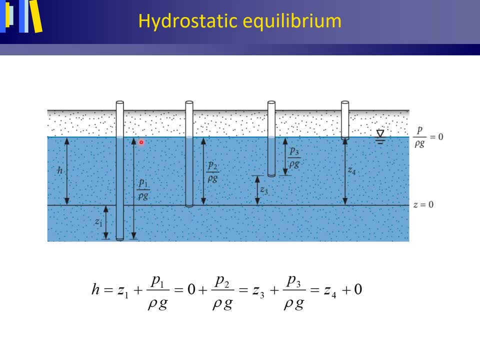 Below the water table, the pressure heads are positive. Above the water table, in the unsaturated zone, the water pressures are negative. Note that under hydrostatic equilibrium conditions, hydrostatisch evenwicht no waterflow, the water table and the hydraulic heads measured in the piezometers have the same level. 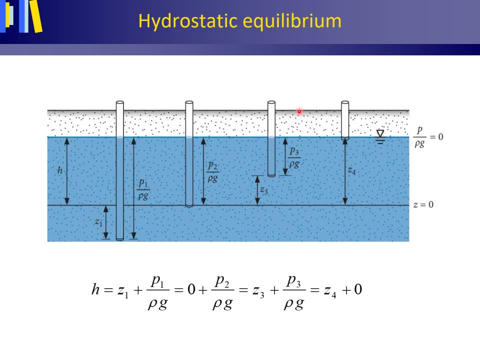 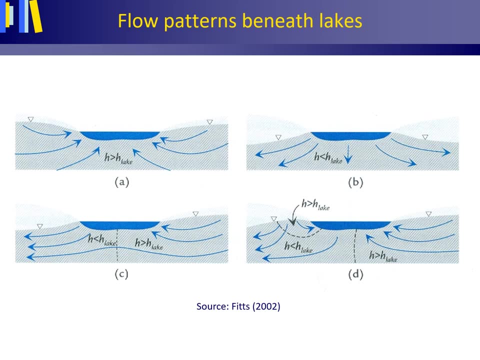 But this is only the case for hydrostatic equilibrium. Flow patterns beneath lakes. These pictures are taken from groundwater science. Groundwater flows from a higher hydraulic head to a lower hydraulic head. We have the landscape, for instance here, and we have the water table. 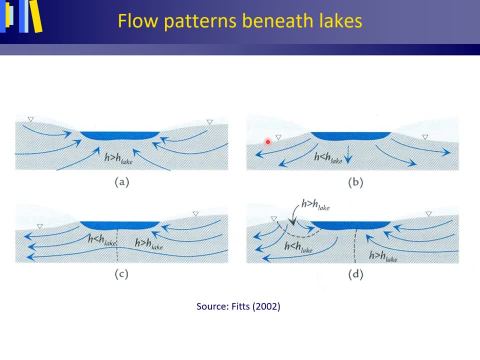 The water table is indicated with this triangle. Here we have a larger hydraulic head in the subsurface than in the lake, the lake level and thus groundwater is discharging into the lake. Here we have the situation the other way around: The hydraulic head in the lake. 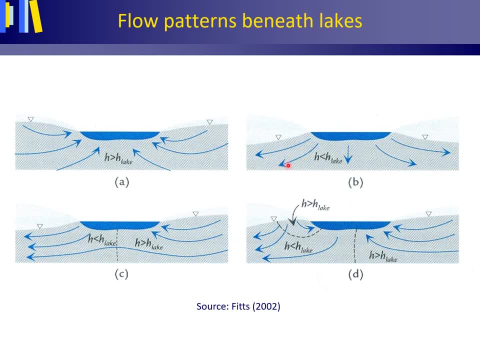 is larger than the hydraulic head in the subsurface and the lake is discharging into the groundwater. Here we have the combination of the two: to the right, groundwater discharging into the lake and to the left, the lake discharging into the groundwater. And here we have yet another combination, to the right again. 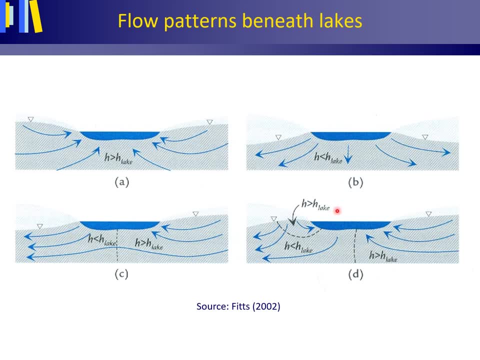 groundwater discharging in the lake and, to the left, the lake discharging in the groundwater. But here we have a local system with a local topographic high and part of the water in this system is discharging into the lake. Let's introduce some of the hydrological terms and 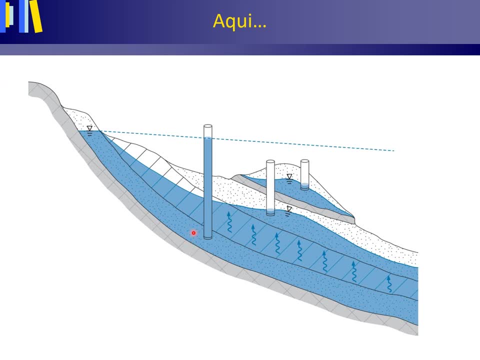 I will use the pointer. An aquifer is a subsurface water storing layer with high water permeability. Permeability is defined for our purpose here in general terms as a measure of the availability of a porous material- soil, sediment or rock- to transmit. 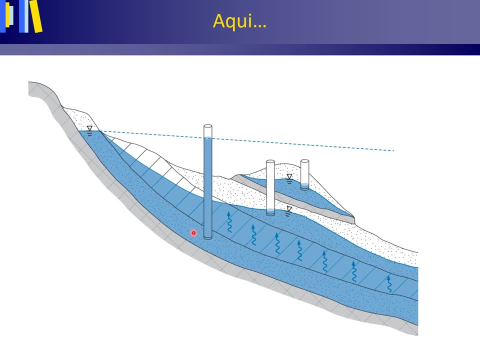 water. An unconfined groundwater has already been defined as groundwater where the water table can establish itself freely. It's also called phreatic groundwater. An aquifer with unconfined groundwater is called an unconfined aquifer, A confining layer. 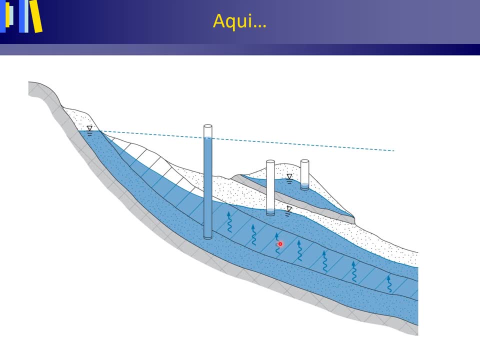 is a subsurface layer with little or no water permeability. Confining layers that totally block groundwater flow- this one or that one- are impermeable layers or aquifuges. Confining layers with low water permeability are called semi-permeable layers, leaky confining layers or aquitards. 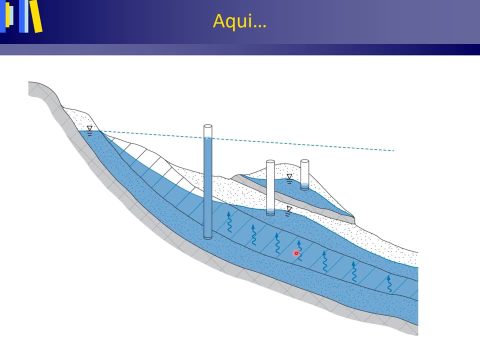 Groundwater captured between two impermeable layers is confined groundwater and the aquifer is a confined aquifer. Ground water captured between two confining layers, one or both of these being semi-permeable- for instance here is called semi-confined groundwater and the aquifer is a 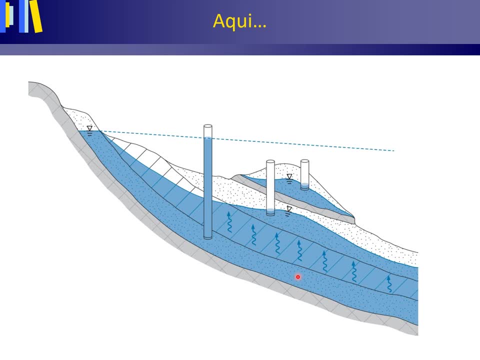 semi-permeable監�💦k is a semi-confined aquifer or leaky aquifer. This figure is a cross-section showing different types of subsurface water storing and water confining layers. The large hydraulic head in the semi-confined or leaky aquifer is caused by a high water. 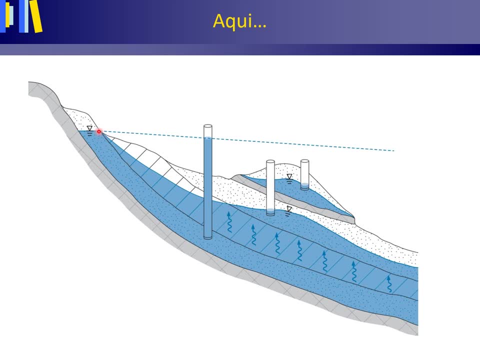 table to the left and by a high water pressure in the aquifer due to the weight of the overlying ground. The semi-confined aquifer is recharged from upslope and its hydraulic head diminishes slightly from left to right. This is due to the friction that the groundwater flow experiences. 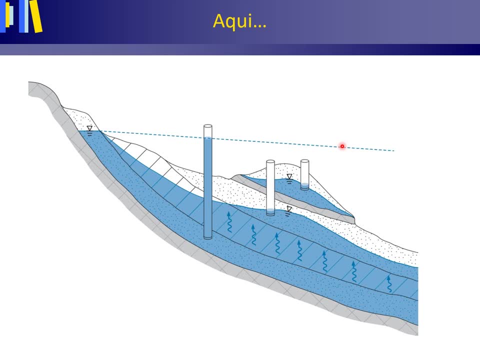 When the hydraulic head of a copper, A confined or semi-confined aquifer, lies above the land surface, as shown here, The groundwater is called artesian. Above the overlying aquitard we observe unconfined groundwater, and to the far right we find 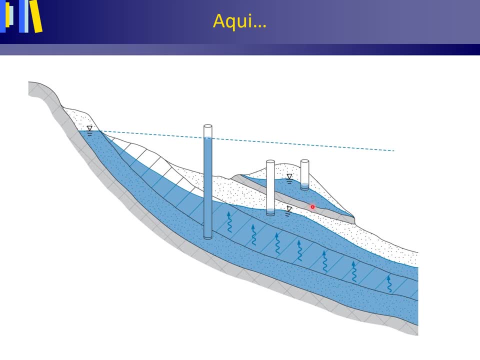 groundwater above an impermeable layer that overlies an unsaturated zone. Unconfined groundwater underlain by an unsaturated zone is called purged groundwater and the water table a purged water table. Note that the hydraulic head is highest in the semi-confined aquifer. 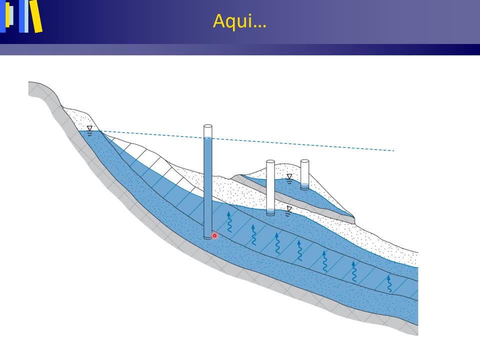 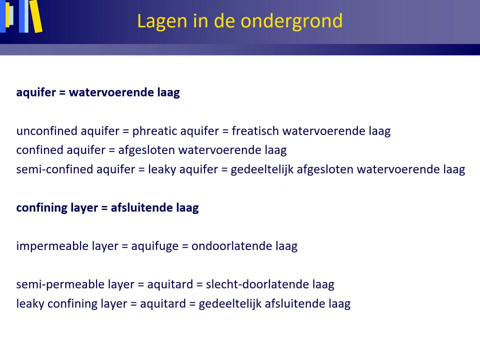 This means that there is seepage groundwater flowing upwards from the confined aquifer through the aquitard that separates both aquifers. And then, for the Dutch speaking students, we have the following terminology for layers in the subsurface: An aquifer is a watervoerende laag. 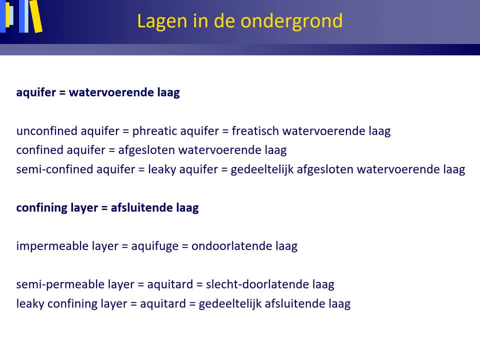 An unconfined aquifer or phreatic aquifer is a phreatisch watervoerende laag. A confined aquifer is afgesloten watervoerende laag. A semi-confined aquifer of leaky aquifer is gedeeltelijk afgesloten watervoerende laag. 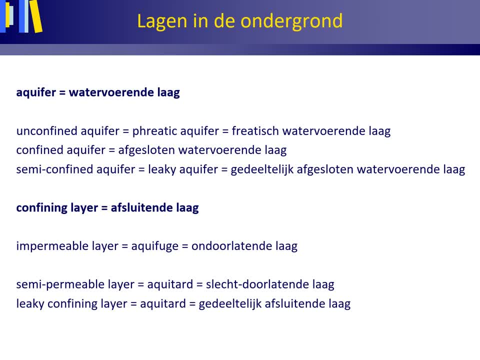 And then for the confining layers, de afsluitende lagen. An impermeable layer or acrifuge is een ondoorlatende laag. A semi-permeable layer or aquitard, is een slechtdoorlatende laag. 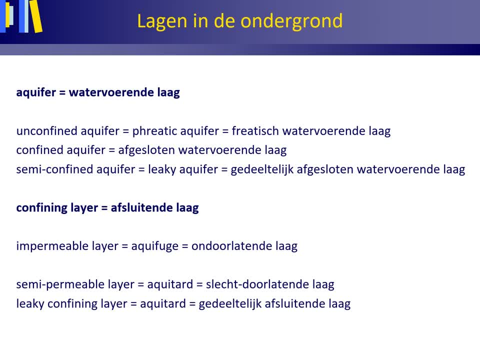 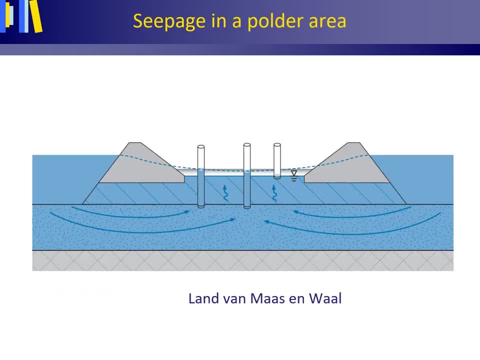 And a leaky confining layer – also an aquitard. The land of Maas en Waal, the Maas River, the Waal River. This figure shows a schematic cross-section of seepage into a polder. The polder is made up of a semi-permeable clay layer and is separated from the rivers. 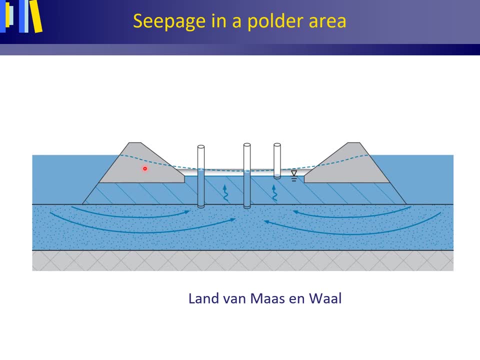 by dikes. Below the clay layer is an aquifer and below the aquifer is an impermeable layer. By pumping any excess water into the river, the water table in the polder, this level is maintained just below the land surface. 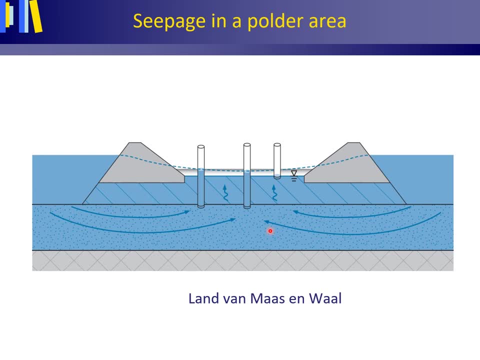 The aquifer below the polder is provided with water from the rivers. as shown by the diagram, Groundwater in the aquifer is confined by an impermeable layer below and a semi-permeable layer above. The hydraulic head in the aquifer beneath the river equals the water level of the river. 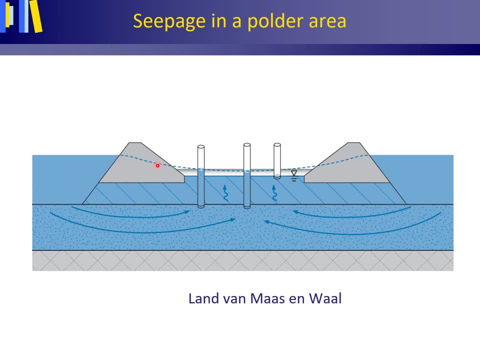 and diminishes gradually to the center beneath the polder. This is due both to the water level and to the level of the river. It is due both to the friction that groundwater flow experiences and seepage through the upper semi-permeable layer into the polder. 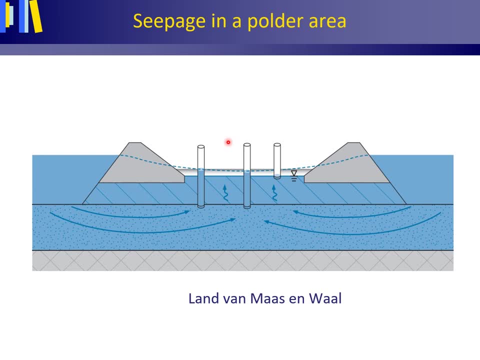 The hydraulic heads in the aquifer are measured in the two piezometers shown on the left. The geographical distribution of the hydraulic heads in the aquifer- the potentiometric surface, as we call it- is presented in cross-section by the broken curve in the upper semi-permeable. 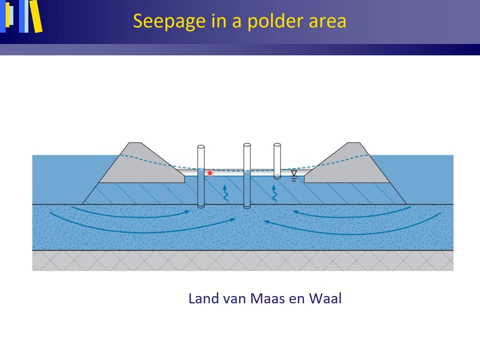 layer. The water level is measured in the upper semi-permeable layer, which is called the log curve. Note that the hydraulic head in the aquifer is everywhere larger than the level of the water table in the polder. This is the level of the water in the polder. 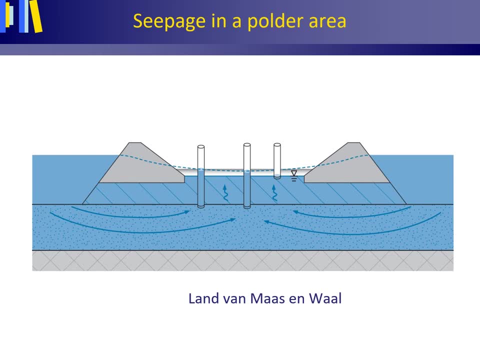 This causes groundwater to seep through the semipermeable layer. Seepage is largest just behind the dikes, where the difference in hydraulic head between the aquifer and the polder's water table is largest, and it diminishes towards the center. 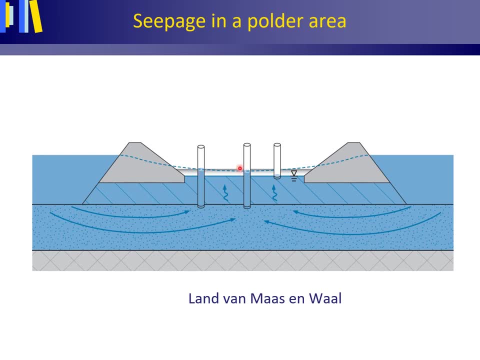 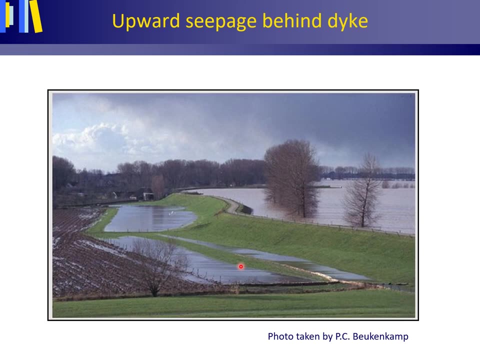 of the polder, where the difference in hydraulic head is smaller. Here we see the result of seepage behind a dike for one of the major Dutch rivers. One of the largest evacuations in recent Dutch history took place in 1995.. 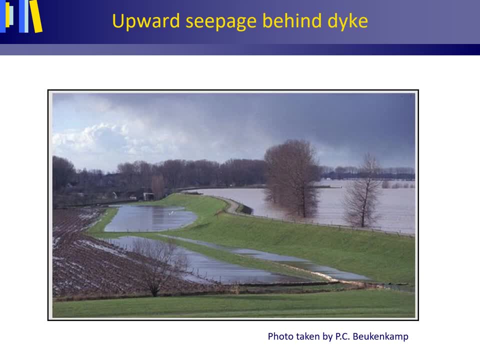 On January 31, 1995 and in the days that followed, 250,000 people were forced to be evacuated, for a period ranging from five days to two weeks, from large parts of the Gelderland River area. This is due to a dangerously high water level of the rivers. 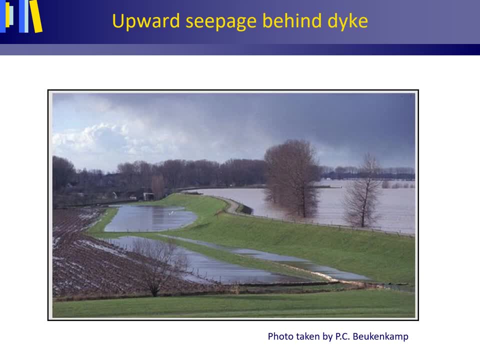 If the dikes would have collapsed, many places in the Betuwe, the Bommelewaard and the Land van Maassenwaal would have been flooded up to approximately five meters. At least the first two floors of many houses would then have been flooded. 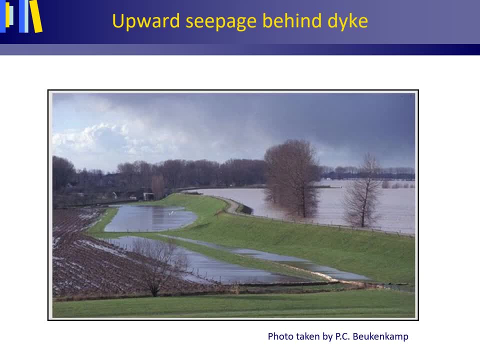 The Dutch dikes are old. They stem from the Middle Ages. Due to this, they are not used. Due to this, they have a low porosity. Had they been new, they would surely have collapsed. As a countermeasure, by placing sandbags in this seepage area, you would increase the 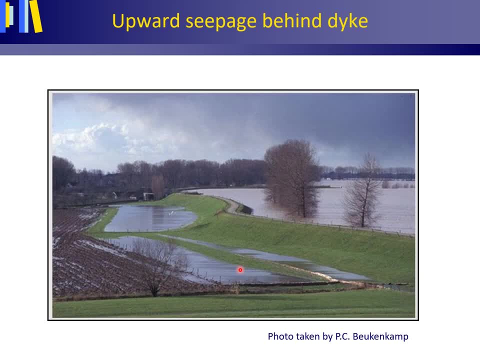 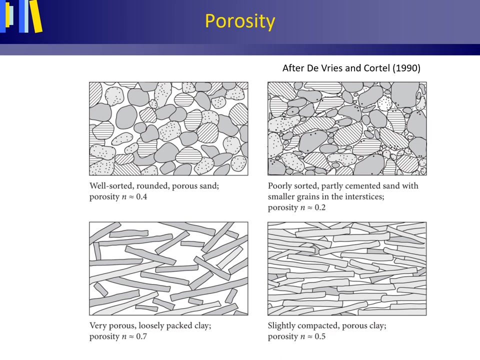 hydraulic head here. By this the difference in river level and hydraulic head here would diminish, causing a lowering of the hydraulic gradient. Then take Darcy's law: This would mean a diminishment of the seepage flow. This figure shows different types of interstices in the subsurface. 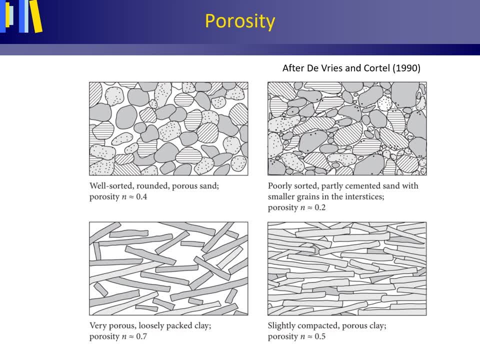 Porosity is the maximum volume fraction of water in the soil. For well-sorted, rounded porous sand, the porosity N is in the order of 0.4,. for a poorly-sorted, partly-cemented sand with smaller grains, the porosity N is in the order of 0.4.. 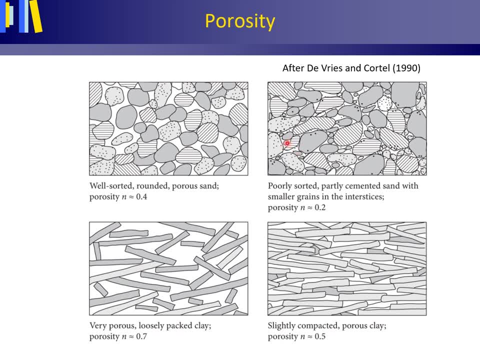 For a poorly sorted partly-cemented sand with smaller grains, the porosity N is in the order of 0.4.. For porous grains in the interstices, the porosity N is in the order of 0.2.. 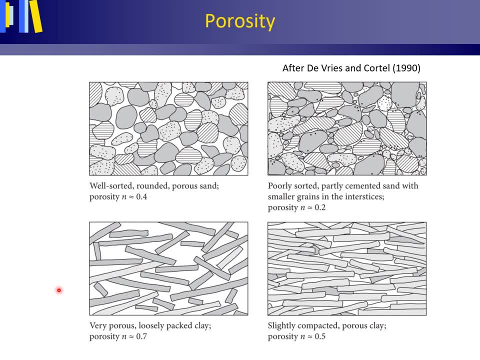 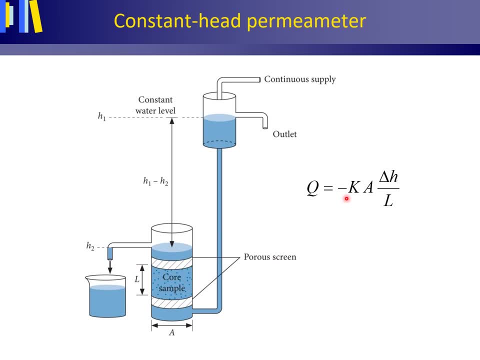 The forces at work in the porous clay, the por頻道 block 0.5 x. the porosity of the KS2F Comes, comes dynamic, dynamic, please, please, please, please, please, please. cubic centimeter core sample. You can establish L and you can establish the value for A. 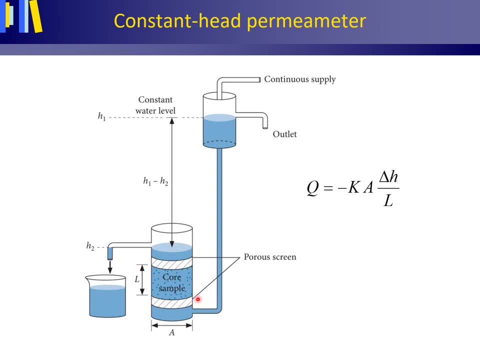 This side of the core sample has a hydraulic head. H1, simply the level of the water here. and then let's take the bottom part of this apparatus as your reference level and this is H1, and the water flowing out of the system as a hydraulic head of. 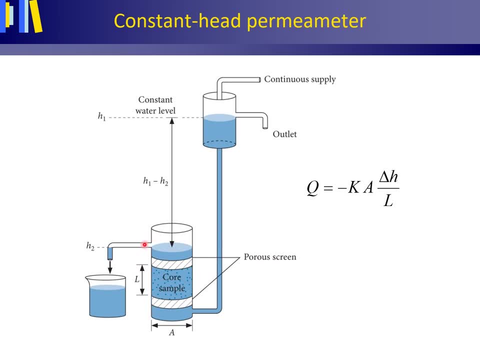 H2.. So the hydraulic head difference H2 minus H1, the hydraulic head to which the water flows minus the hydraulic head from which the water flow dispatches- H2 minus H1, is a negative number. These are all positive numbers. We have a minus sign here. 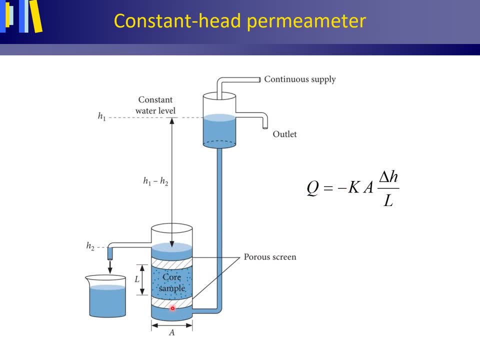 so your volume ratio is negative. The volume flux here is a positive number, and that's correct because the water is flowing upwards. You can simply determine this volume flux by simply catching the water here, and then you can determine the volume per unit time. So you know all the variables and you can simply 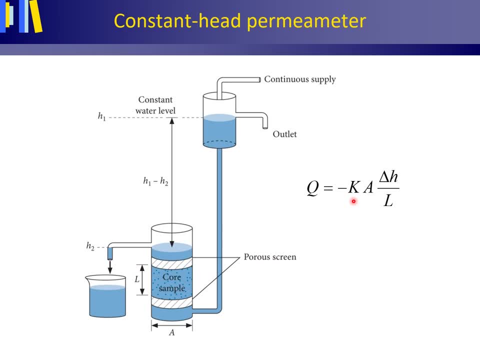 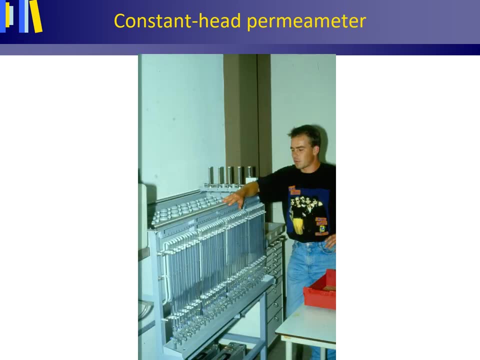 figure out what your saturated hydraulic conductivity is by using Darcy's law. Here we have a constant head permium meter in the laboratory with a young PhD student- now professor Mark Bierkens at our institute, standing next to it, As you can see your 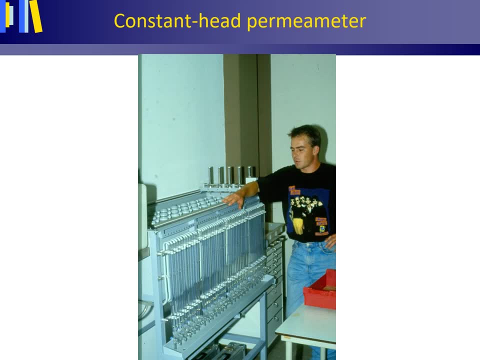 measurements are not limited to one subsoil core sample, but you can insert many of these. You can determine the volume fluxes here and then, simply by applying Darcy's law, you can figure out what the saturated hydraulic conductivities for these subsoil core samples are. 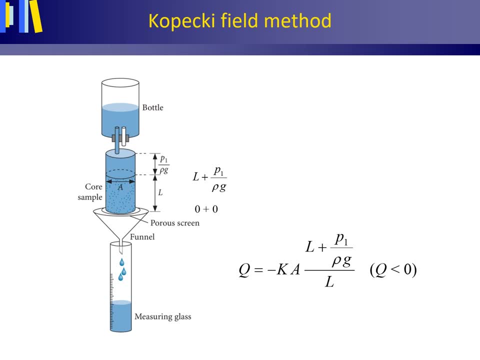 Another measuring technique, also involving the use of one or more core samples of the subsoil, but usually performed in the field or during field work, is the Kopecky field method. A bottle is filled with water and closed by a cork with two open tubes. 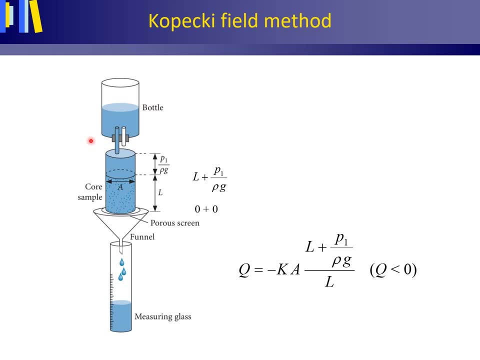 The bottle is then turned upside down and water is fed onto the subsoil sample. as shown in this figure, The short tube lets the air in, while the larger tube lets the water out When the water above the subsoil core sample reaches the outlet level of the larger tube. 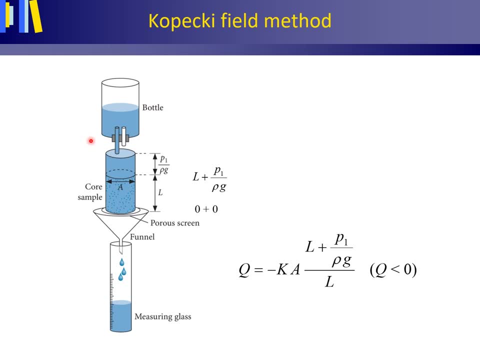 the water flow from the bottle is temporarily halted. In this way, a constant water level above the subsoil core sample is created, with water infiltrating from this water layer into the subsoil core sample. After the subsoil core sample is water saturated. 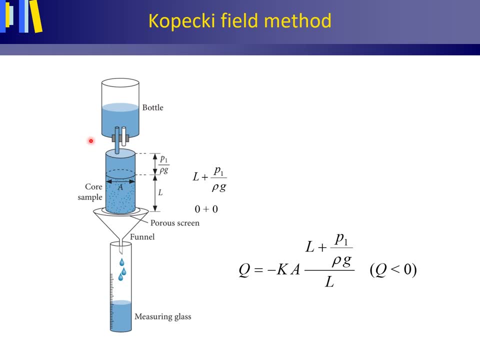 and as soon as the volume flux Q attains a constant value, the hydraulic conductivity of the subsoil sample can be determined, again by application of Darcy's law. Note that the water flow from the subsoil core sample is downward and that Q, the volume flux, thus has to be assigned. 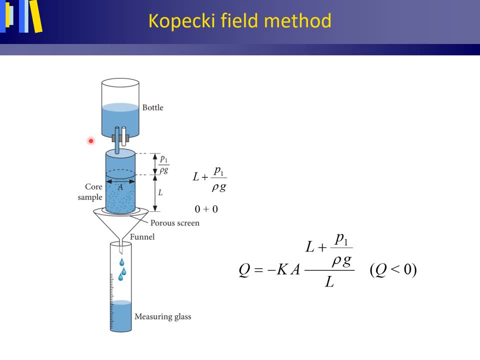 a negative sign As outflow from the subsoil core sample is under existing air pressure. the pressure head at the water dispatching end of the subsoil sample equals zero meter If we take the bottom of the subsoil core sample as the reference. 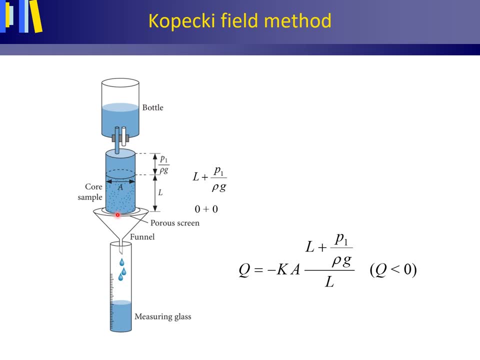 the hydraulic head at this water dispatching bottom end of the subsoil sample thus equals an elevation head of zero meter plus a pressure head of zero meter, totaling zero meter On the water receiving upper side. the hydraulic head equals an elevation head of L plus a pressure head. 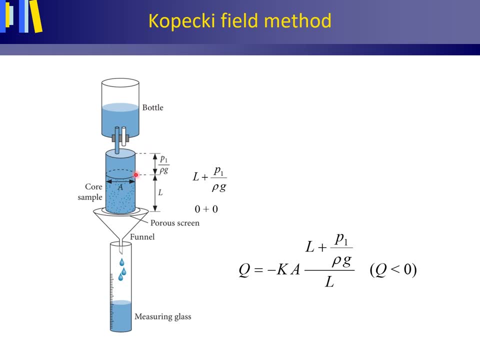 of P1 divided by L, Both L and P1 divided by rho g being positive numbers. The difference in hydraulic head thus equals zero, minus in between brackets, L plus P1 divided by rho g. close the bracket. so zero minus L minus P1 divided by rho g, The hydraulic gradient. 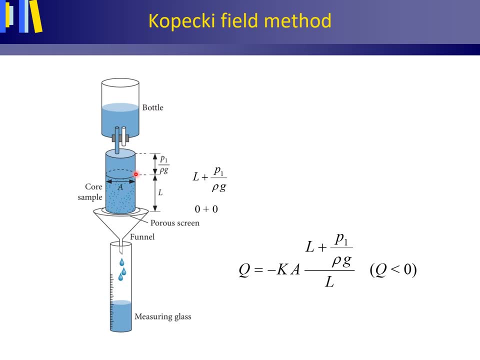 and the pressure head have the same number. The difference in hydraulic head is zero minus L times the pressure head. In the D'Ascen equation you get a deviation: The difference in hydraulic head decibed by the distance. The distance is 0 minus L. Insert all of this in D'Arcy's law and 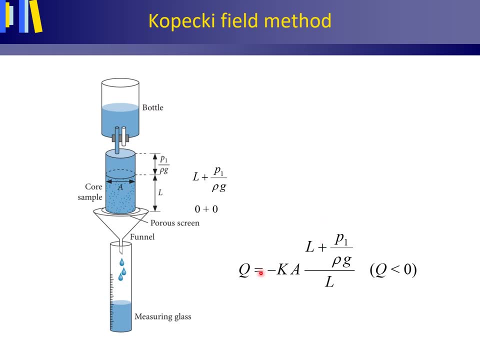 you will get this equation. Please note that, because the water is flowing downwards, that your Q, your volume, flux, is a negative number, And please do not learn this formula by heart, but make sure that you can obtain a negative quantity. You can derive this simply by rewriting Darcy's law, as I just explained. 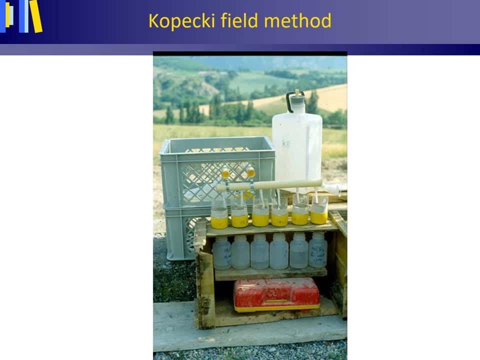 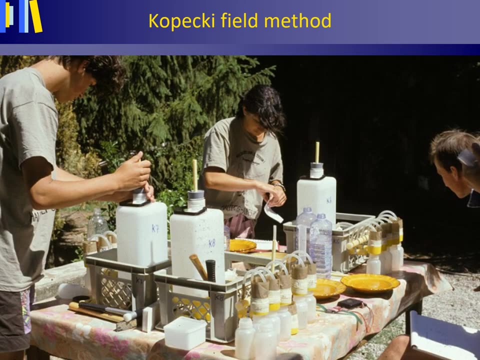 And this is just to give you an impression of the Kopecky field method, again in our fieldwork area in the Autalps in France. And this is yet another picture taken during that same fieldwork, also of the Kopecky field. 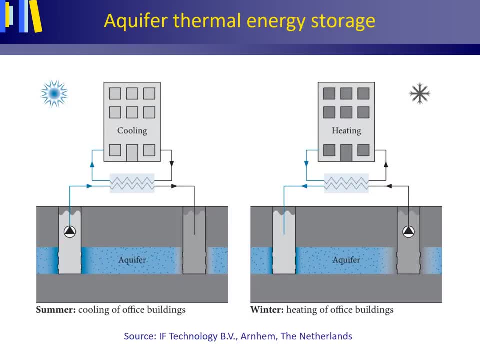 method. This figure shows the principle of aquifer thermal energy storage. The left part of the figure shows the summer situation where cold groundwater is pumped out of an aquifer. to the left, The cold water is used for cooling a building using its air conditioning system via a heat. 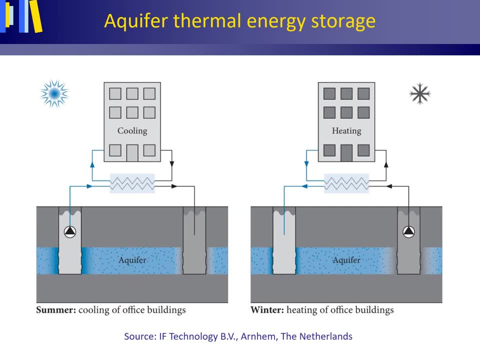 exchanger. Note that the groundwater that has warmed up during the heat exchange process is returned to the aquifer In winter. the operation is reversed. The right part of this figure shows the warm water which infiltrated during the summer now being pumped out. 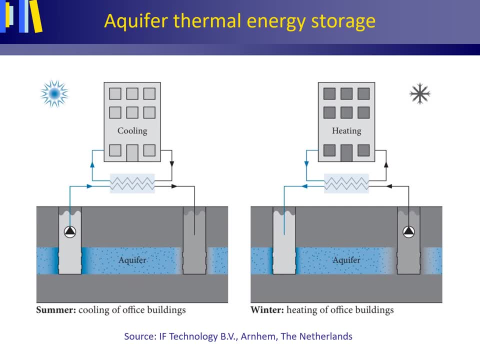 The warm water is used for heating the building using its central heating system via a heat exchanger. Note that the groundwater that has cooled during the heat exchange process is again returned to the aquifer now for later use in the summer, and so on. 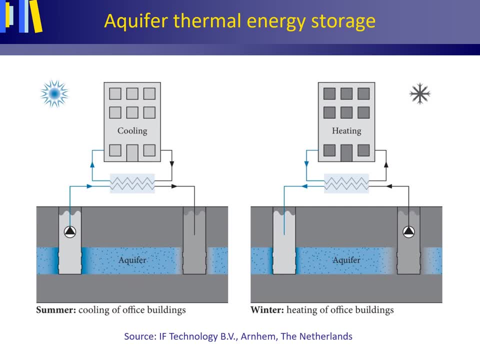 Groundwater holds its temperature, The thermal conductivity of aquifers is low and groundwater flow is slow, as we have calculated, causing aquifer thermal energy storage to be an effective technique for both the cooling and heating of buildings, replacing part of the electricity demand in doing so, and thus 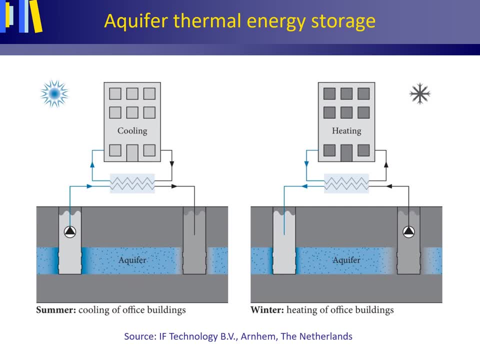 also reducing possible burning of fossil fuels and CO2 emissions into the atmosphere. At Utrecht University, near the Weening-Meiners building, we have an aquifer thermal energy storage project in use. The saturated hydraulic conductivity K, as used in Darcy's law, strongly depends on the 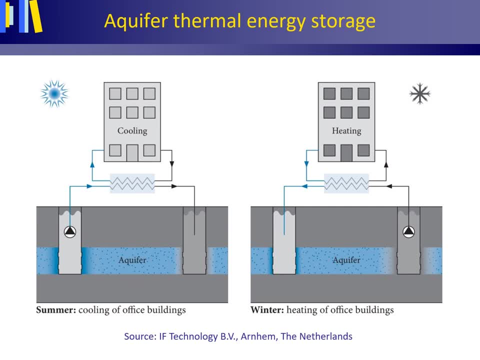 groundwater's temperature. Therefore, calculations of the volume flux Q and the effective velocity of groundwater in aquifers used for thermal energy storage can be used to calculate the volume flux Q and the effective velocity of groundwater in aquifers used for thermal energy storage. 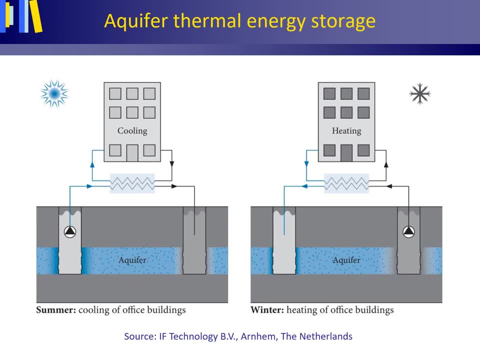 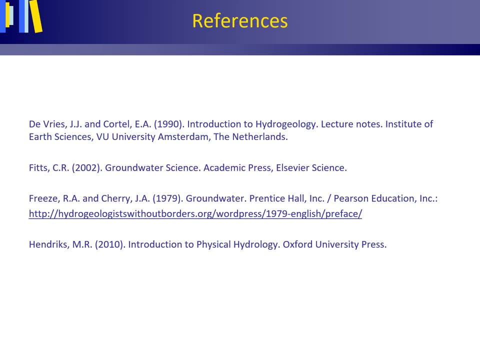 as shown here, We have come as far as section 3.7 of my book and you can now make all the exercises up to exercise 3.7.5.. Good luck. 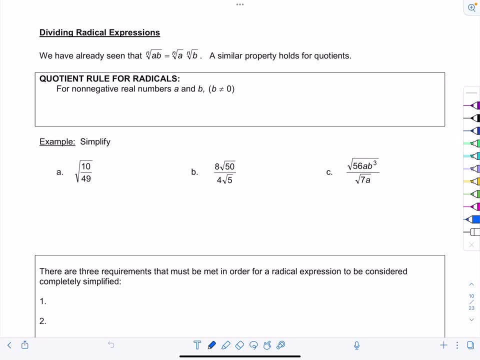 Hey everyone, welcome to Math TV with Professor V. This is video lecture number 35 for intermediate algebra, and we're going to talk about dividing radical expressions. Now, building on the last video, we looked at the product rule for radicals, So we've already seen that if you have the nth. 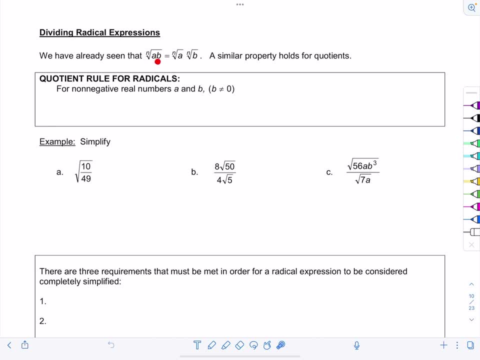 root of a- b. so you have a product under the radical sign in the radicand. you can break it up and write it as nth root of a times nth root of b, as long as a and b aren't negative And a. 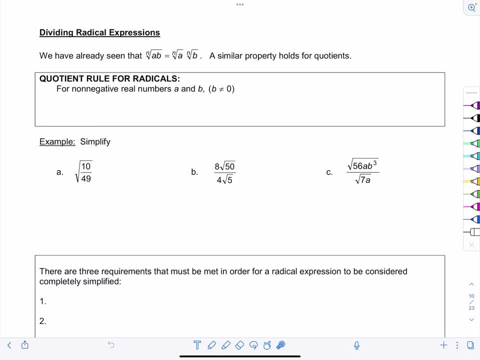 similar property holds for quotients. So here's the quotient rule for radicals. Again, for non-negative real numbers a and b, we have the following: that the nth root of a divided by b is equal to the nth root of a over the nth root of b. 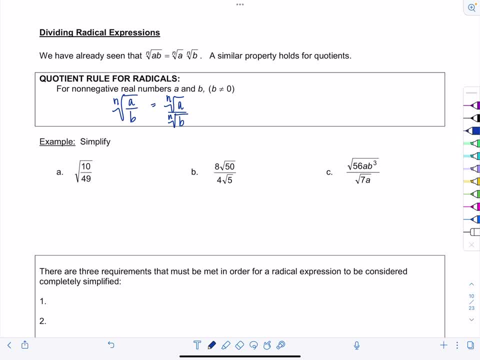 So they're all the same thing. So we're going to look at the product rule for radicals. So we're going to look at the product rule for radicals. So we're going to look at the product rule for radicals. Basically, you can split up a radical sign over division as well, So let's use that rule to. 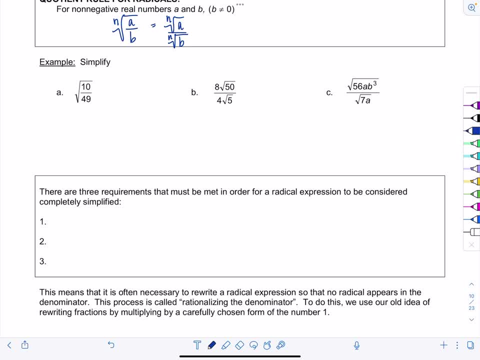 simplify some of the following radical expressions. First one: we have square root of 10 over 49. So split them up, give them each their own radical square root of 10 over square root of 49. And then let's check: can this be simplified further? Because remember, in the last lesson, 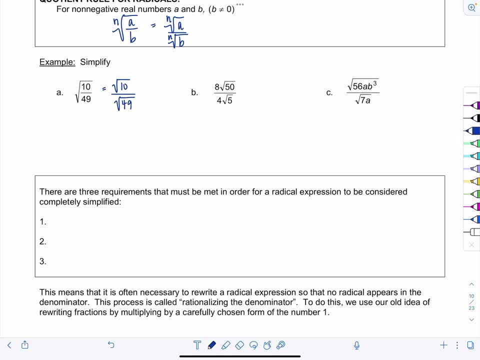 we learned how to simplify radicals. Well, square root of 10,. no, that doesn't simplify No perfect squares divide evenly into 10, but square root of 49 is 7.. So I'm going to box this and call it a day. There's our answer. Okay, It's an ugly little box and I. 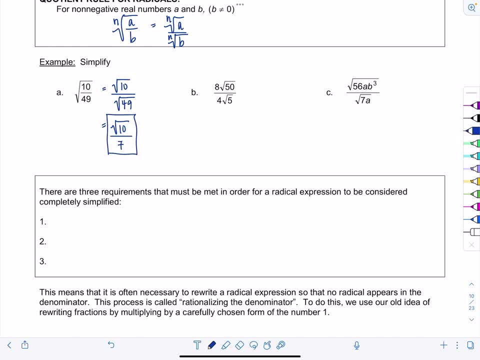 don't like it? All right, we're just moving on. Okay, b 8, rad 50, over 4, rad 5.. So now we're going to go the other way. actually, You see how we already have two radicals. Well, we're going to.